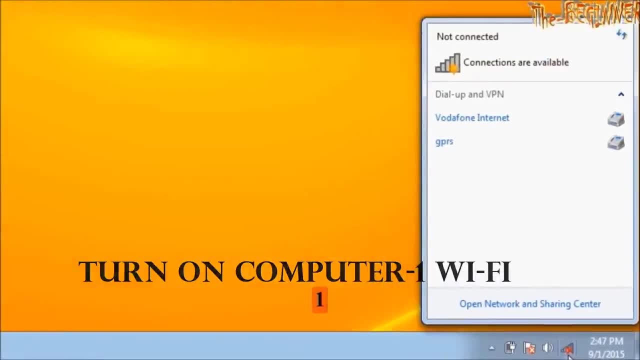 Now turn on your computer. 1 Wi-Fi switch. Mostly your Bluetooth and Wi-Fi switches are same. See here. Since nearby I have no network connection, so nothing is visible here. These two are USB modem connection, not Wi-Fi. Leave it. 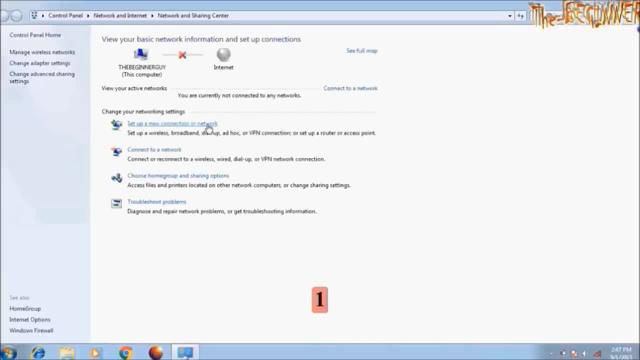 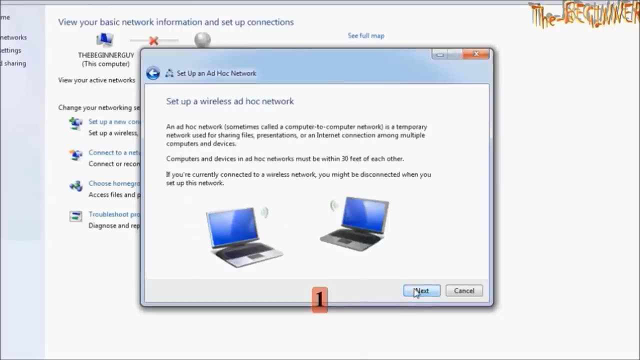 Open network and sharing center. Click on setup a new connection or network. Go down and choose setup a wireless adhoc network and click on next. Then next choose any network name. Security type should be WPA2, which is Wi-Fi protected access. 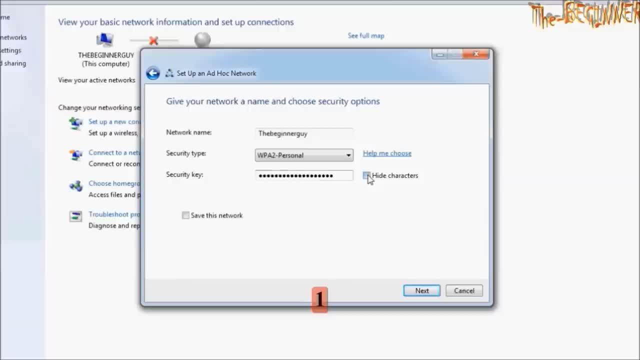 Don't change it and choose password of minimum 8 character. You can hide or show character from here. Save this network and click next. Now I have successfully created a adhoc network. Close it and come to the computer. 2. Turn on its Wi-Fi switch: Click here. 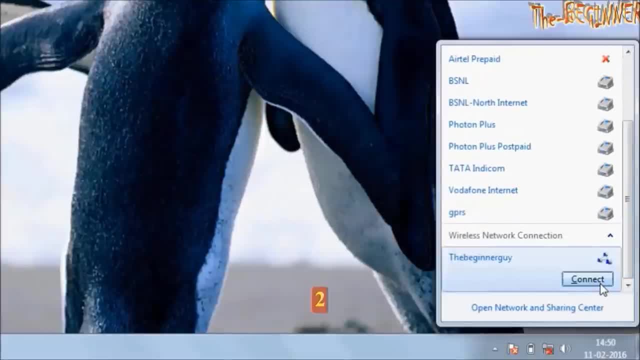 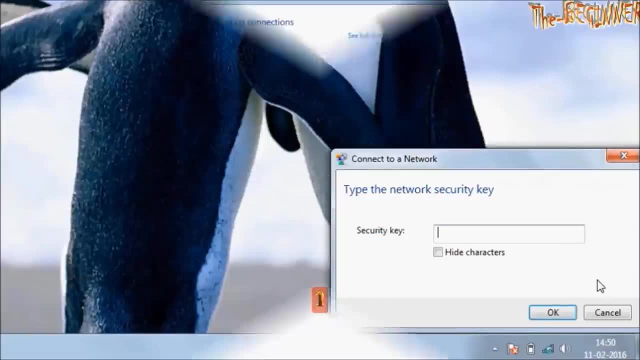 See it is showing wireless network connection. The beginner guy Click here and click on connect. It will ask password. Suppose I have forgotten the password which I have created, Then what should I do? So come back to the computer 1 and click here: manage wireless networks. 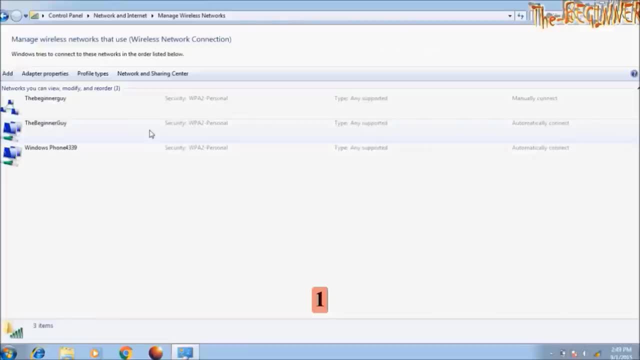 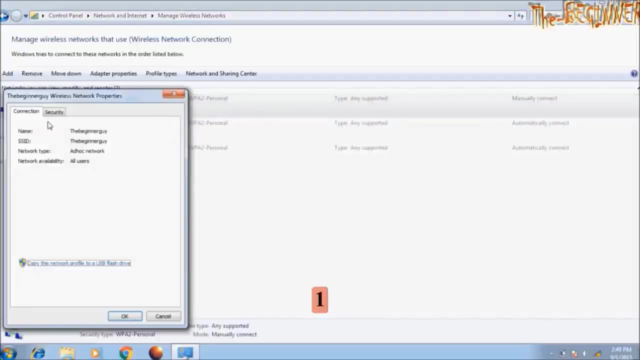 I may confuse here with the name, since I have created adhoc network. So this 3 computer is symbol of adhoc network. So choose it Right click here and click on properties. Go to security and click here. You can now see the passwords. 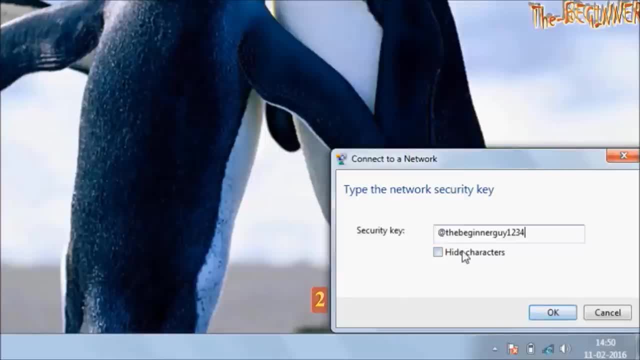 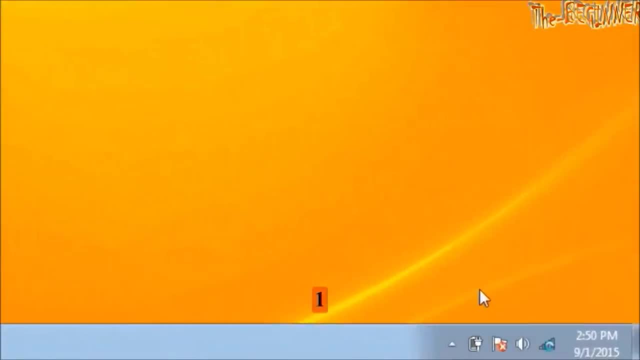 Now back to the computer. 2. Fill password here And then OK, It will connect in few seconds. Come back to computer. 1. See, it is connecting. So I have connected both computer. So what next? Let's see. 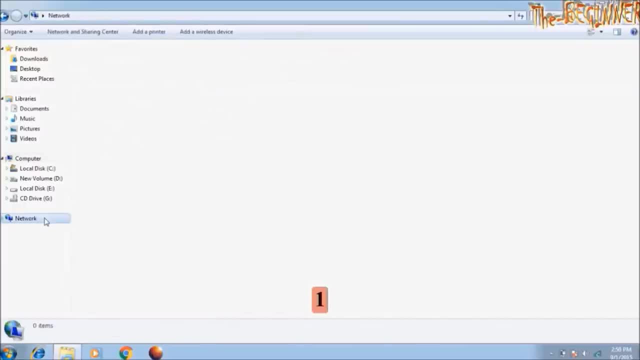 Go to my computer and click on network Refresh here. Wait for seconds And here it comes. The beginner guy is the computer 1 itself. In network section it shows other computer along with this computer. This shivhp is computer 2.. 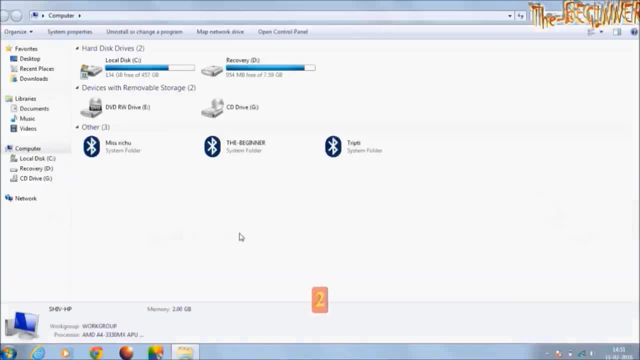 You can verify it in computer 2.. Open my computer, right click here and click on properties. See this shivhp. it is computer 2.. Also in computer 2, you can see computer 2 itself. that is shivhp and other computer. that is computer 1, the beginner guy. 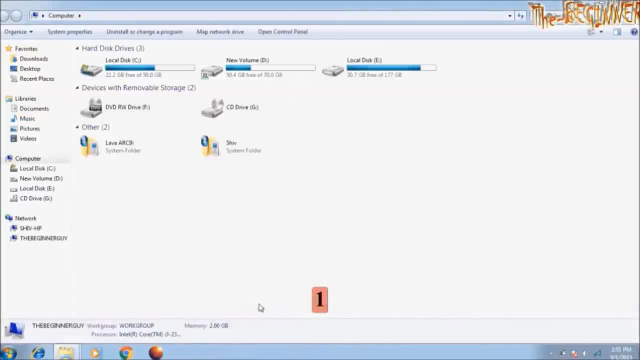 Now come back to the computer 1.. You can cross check that computer 1 is the beginner guy. I have connected both computer. So in network section both computer names are visible. Now open network and sharing center. Click on change advanced sharing setting. 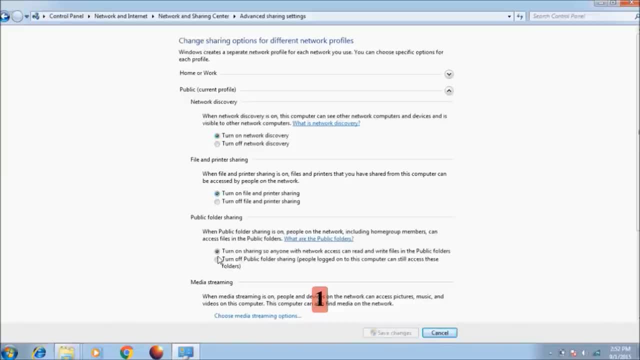 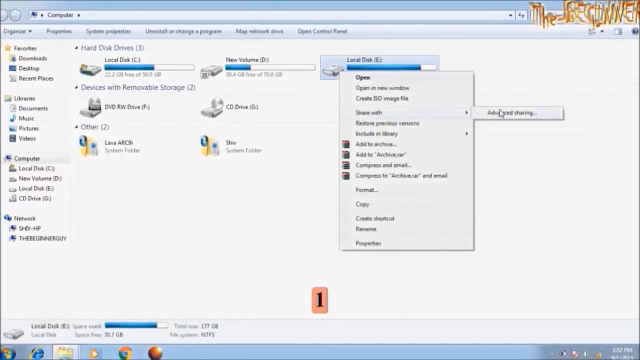 To share files, you have to turn on all these and then click on save changes. Now I am going to share files between these two computer. Right click on drive share with advanced sharing. Click on advanced sharing Check. share this folder. 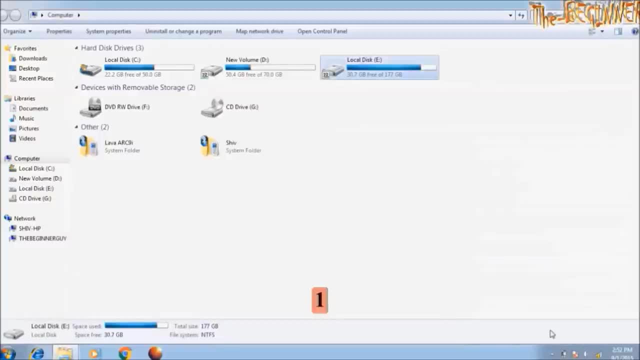 Then apply, then ok, Close it. This symbol is showing that this drive is shared. D drive is also shared. Now come back to computer 2.. Here C drive is shared. I am in computer 2 and I am going to open computer 1.. 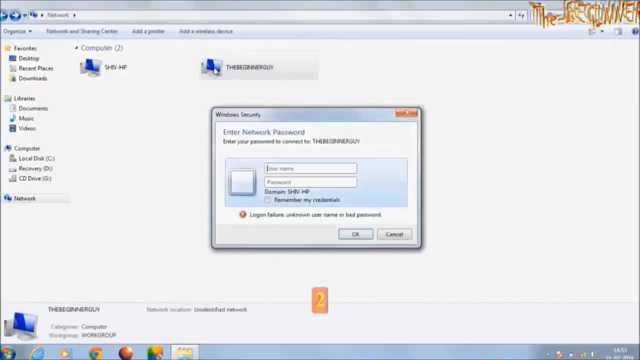 That is the beginner guy. So double click on the beginner guy. It will ask username and passwords. Listen, computer name and username is two different things. Your computer has its name, like shivhp, the beginner guy, and this computer may have one or more users. 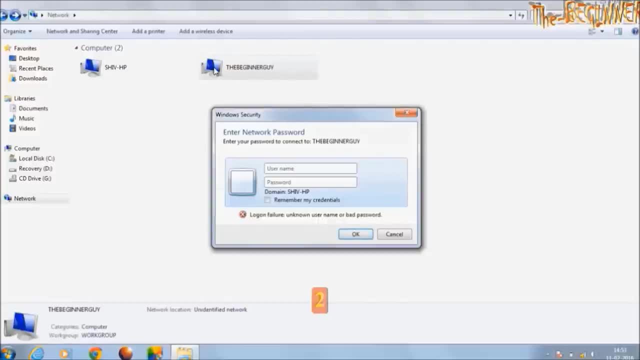 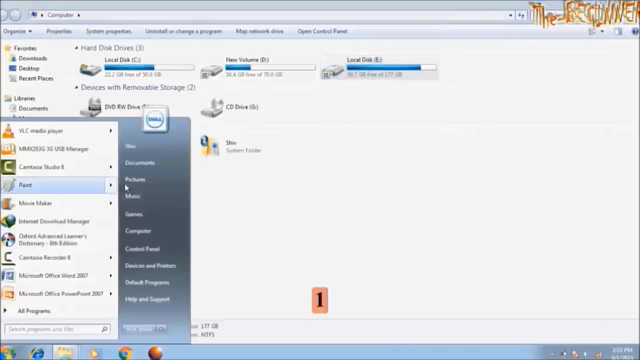 When you open your computer and where you fill passwords, that name mentioned is user. That username and password is asking. here You can check username in computer 1 from here. This is username shiv. Please don't confuse with the names Both. computer is mine. 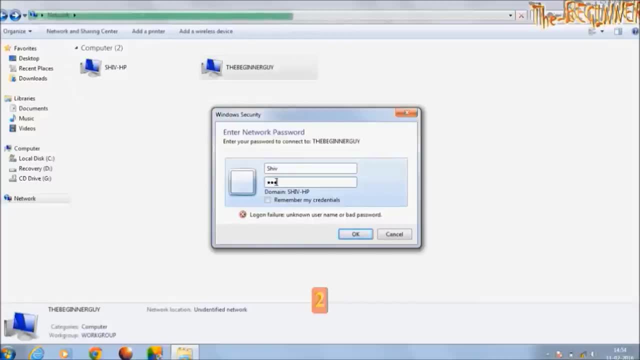 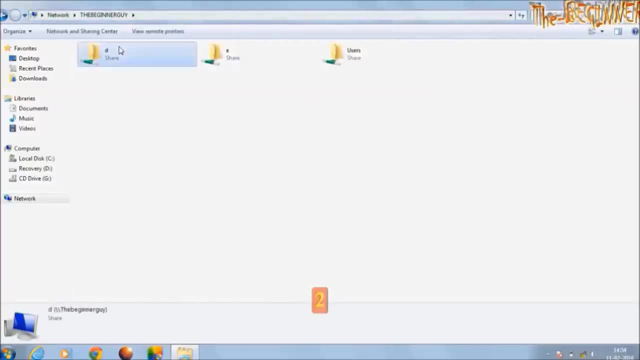 So names are mostly same. So fill username and password of computer 1 here, Then press ok. See, I can view D drive, E drive of computer 1 from computer 2.. Open D drive. You can confirm it from computer 1 also. 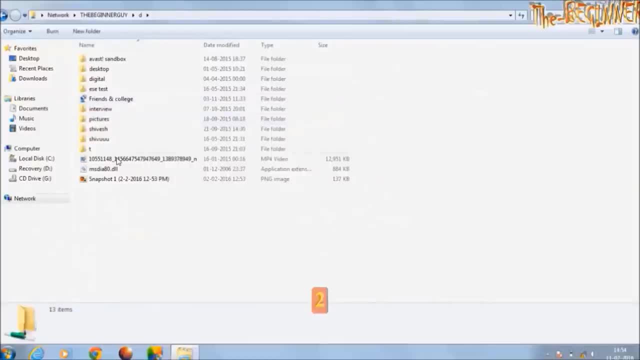 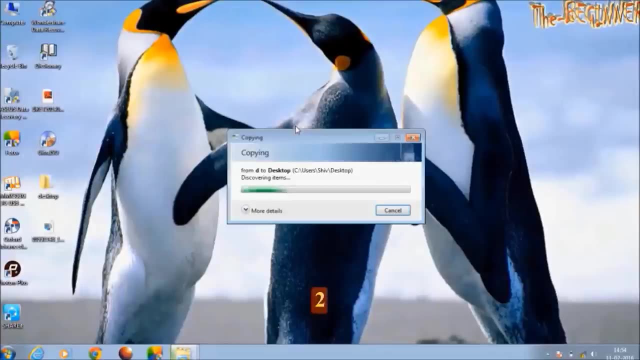 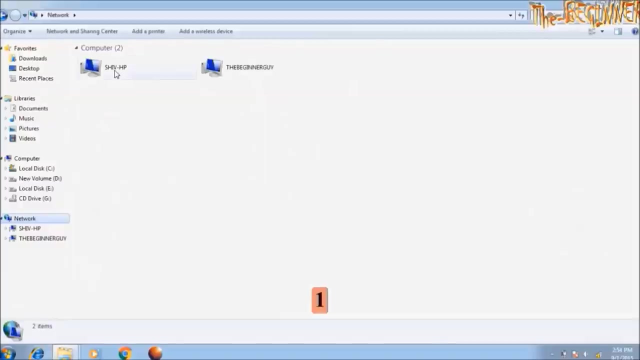 That files are same. So here you can copy any files and paste anywhere in computer. 2. Now back to the computer. 1. From here also you can open computer. 2. That is shivhp Username and fill passwords. 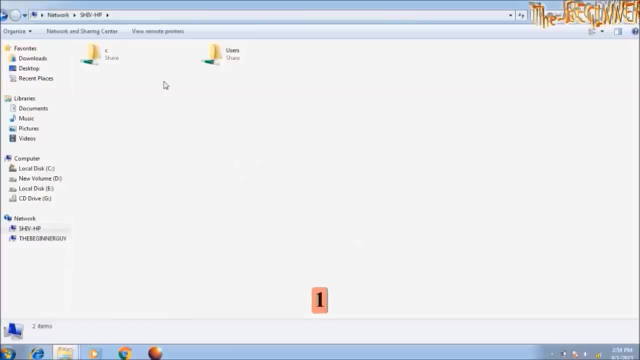 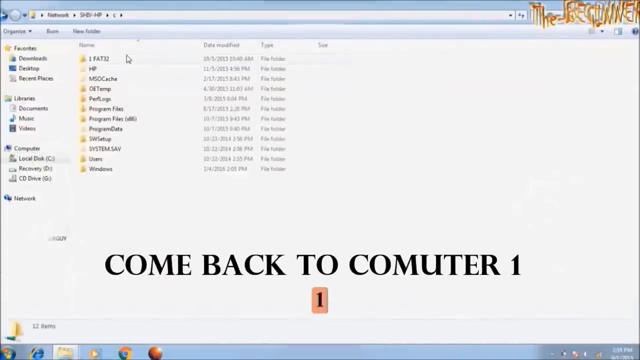 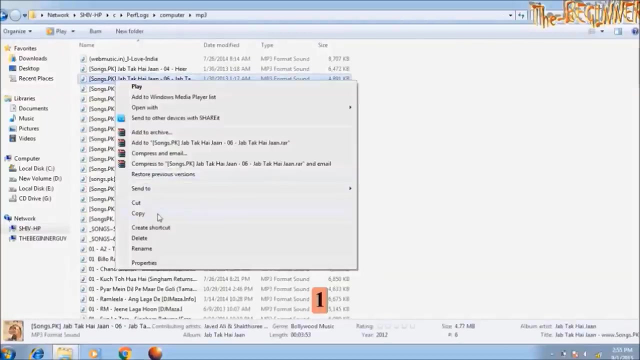 Then press ok. See C drive which was shared in computer 2. You can verify again in computer. 2. The files are same From here also you can copy files and paste anywhere. One more things: When both computer gets connected.